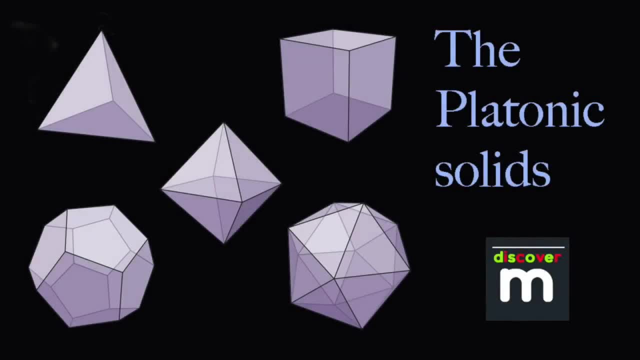 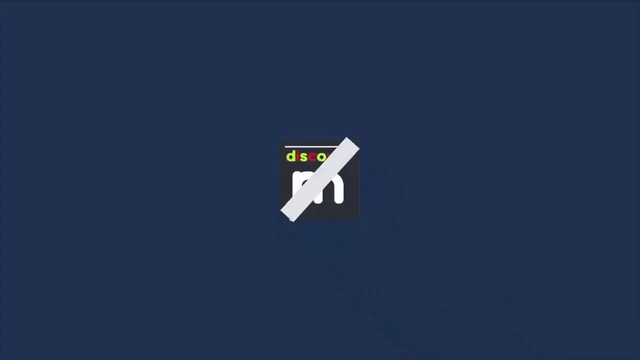 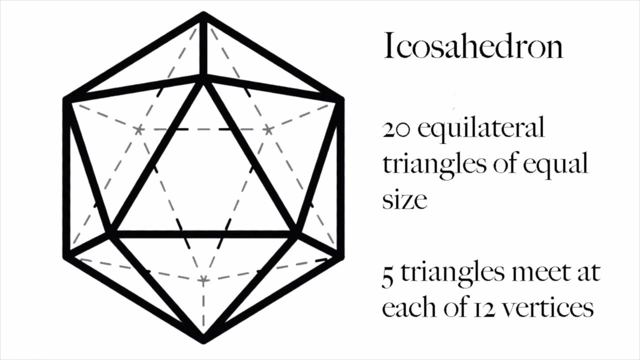 Today I'm going to be talking about the Platonic solids, special shapes in three dimensions that have been known about since antiquity. First of all, what is a Platonic solid? It's a regular convex polyhedron. So what does? 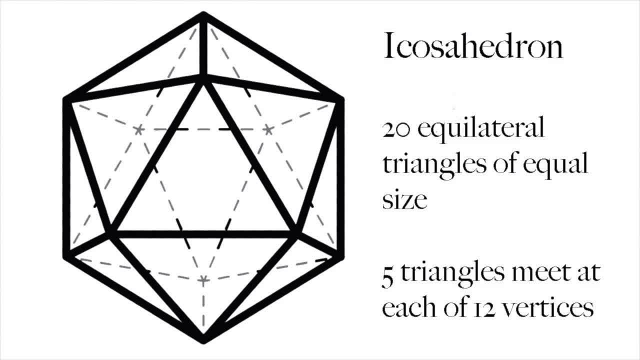 that mean? Well, a polyhedron is a three-dimensional shape with flat sides. Regular means that all the sides are the same shape and size, and convex means that any two points on the surface can be connected by a line that doesn't cut through the surface. There are exactly 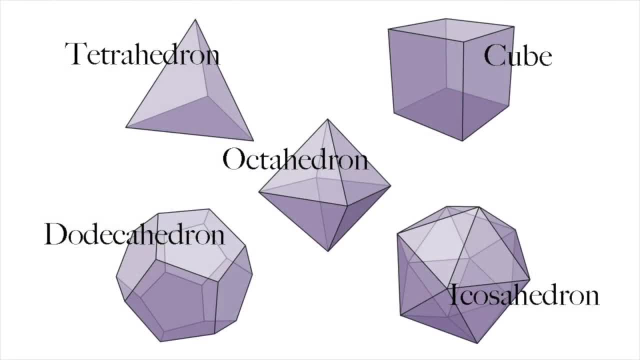 five platonic solids: The tetrahedron, the cube, the octahedron, the dodecahedron and the icosahedron. These have got four, six, eight, twelve and ten. It's easy to see why there can't be any more than the five platonic solids, At least three. 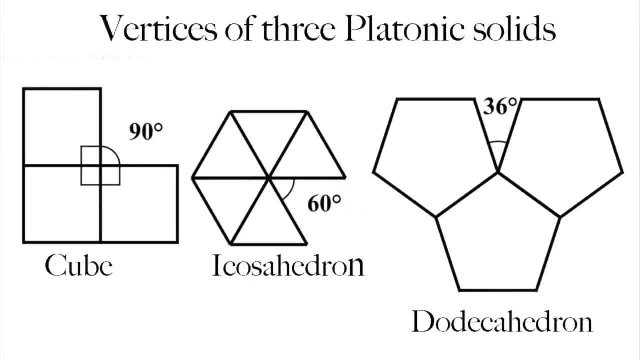 faces have to meet at each corner or vertex in order to make a closed 3D shape. And when you add up the internal angles that meet at a vertex, it must come to less than 360 degrees, otherwise the shape would just flatten out. A regular or equilateral triangle has internal 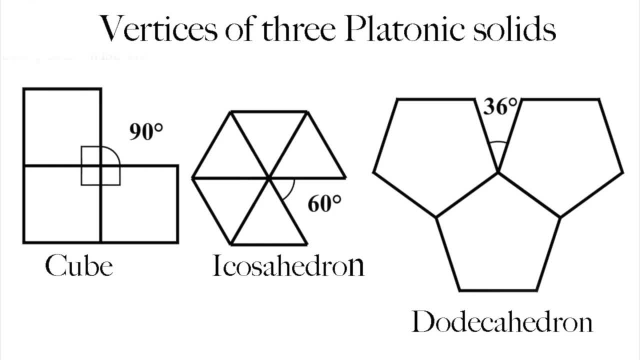 angles of 60 degrees. So you can satisfy the conditions for a platonic solid by having three, four or five regular triangles meeting at each vertex leading to the tetrahedron, the octahedron and the icosahedron. The internal angles of a regular quadrilateral or square are 90 degrees. 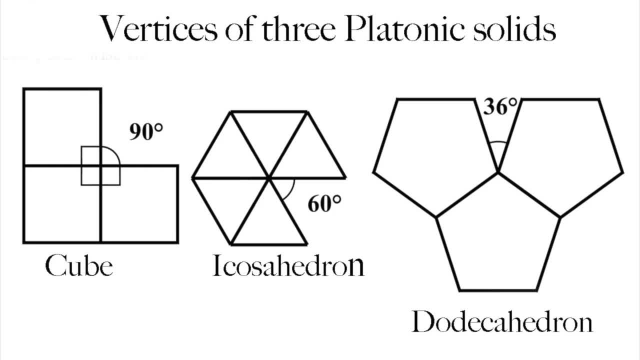 So you can make only one platonic solid from squares: the cube, with three squares meeting at each vertex. The internal angles of a regular pentagon are 108 degrees. So again, you can make only one platonic solid using pentagons: the dodecahedron. 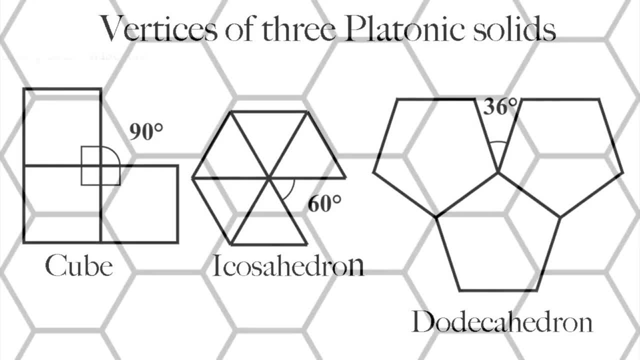 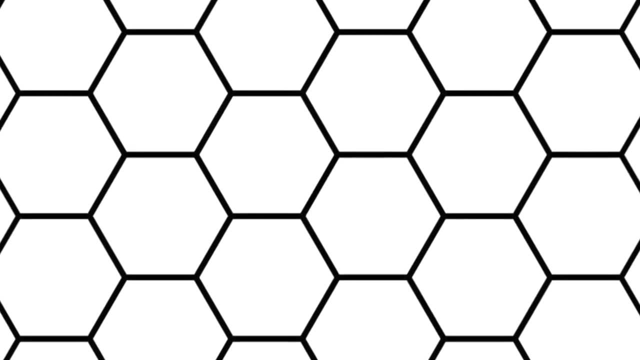 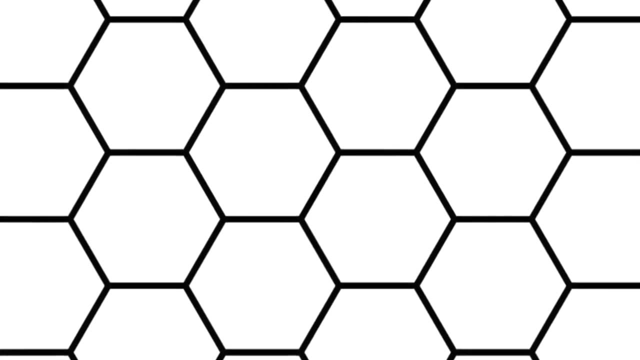 And there you have it, the five platonic solids. You can't make a regular convex polyhedron that has hexagonal faces, because a hexagon has internal angles of 120 degrees. So if you make three regular hexagons meet at a point, they'll just form a flat surface, not.